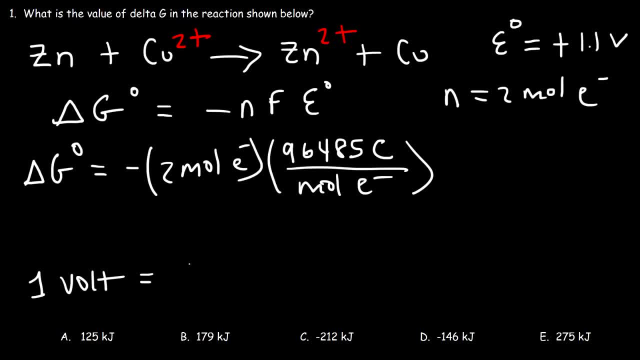 Now you need to know that 1 volt is 1 joule per coulomb. Joule is the unit of energy and work, Coulomb is the unit of charge. So 1 volt relates potential energy to charge. It's 1 joule per coulomb. 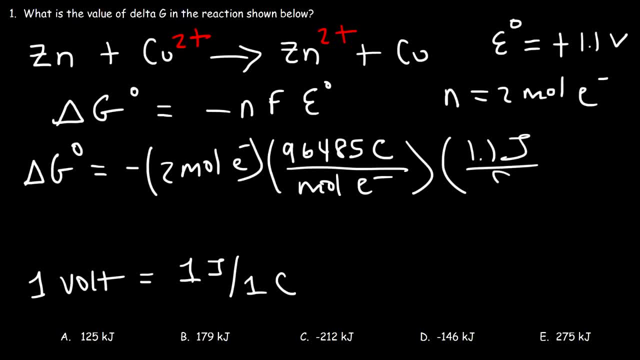 So we have 1.1 volts or 1.1 joules per coulomb, And so we can see that the unit moles of electrons will cancel And the unit coulombs will cancel, And so we're going to get delta G in joules. 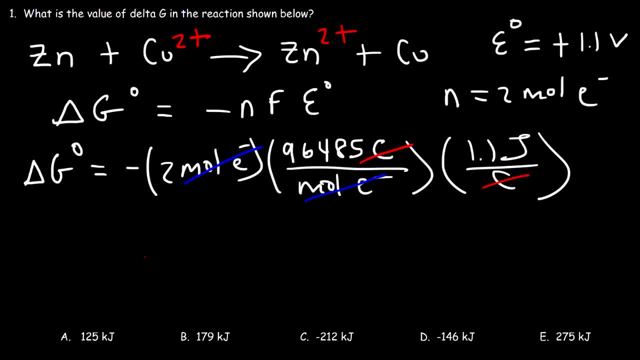 So negative 2 times 96,485 times 1.1.. That's equal to negative 212,267 joules. Now let's convert that to kilojoules. One kilojoule is equal to 1,000 joules. 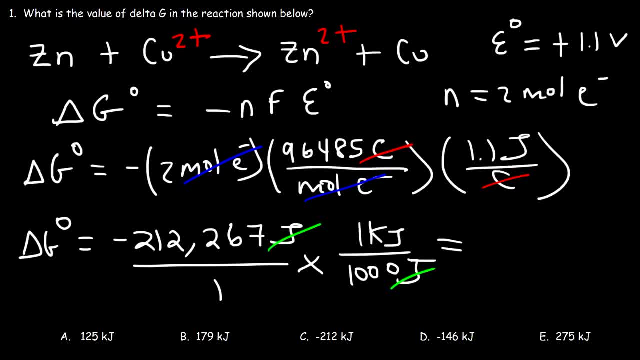 And so we can see that these units will cancel, And so this is going to be approximately negative 212.267, if you want to add that, kilojoules, And so that's the answer for the problem. So this correlates to answer choice C. 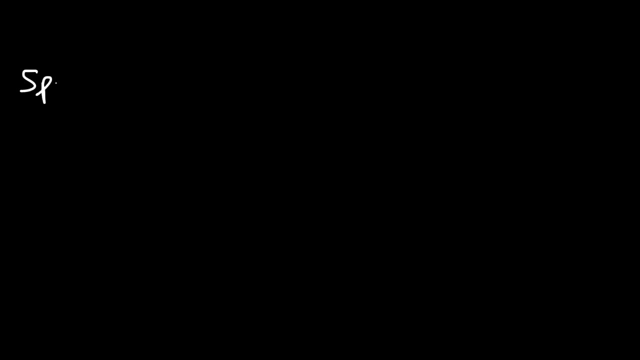 Now here's a question for you: For a spontaneous chemical reaction, what is the sign of the cell potential and also delta G? And what if the reaction is non-spontaneous And also if it's at equilibrium? For a spontaneous reaction, delta G is negative. 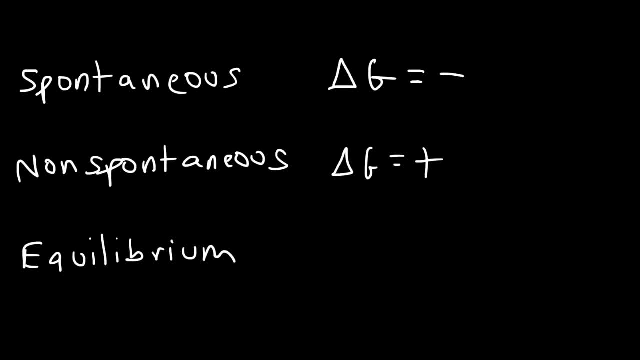 And it's positive if the reaction is non-spontaneous in the forward direction. If it's at equilibrium, delta G is zero. Now we know that delta G is equal to negative NFE. So because of the negative sign, delta G and the cell potential have opposite signs. 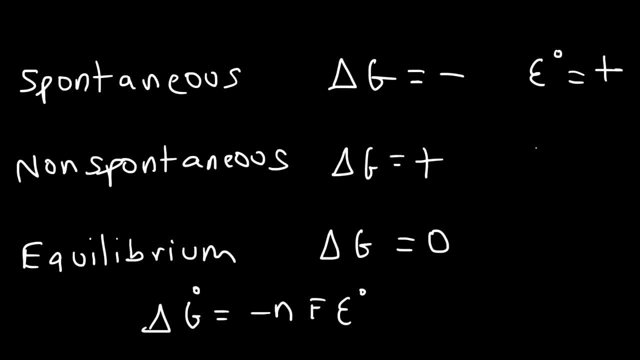 So if delta G is negative, the cell potential will be positive, If delta G is positive, the cell potential will be negative, And if delta G is zero, the cell potential is zero. So for a spontaneous process the cell potential is positive. 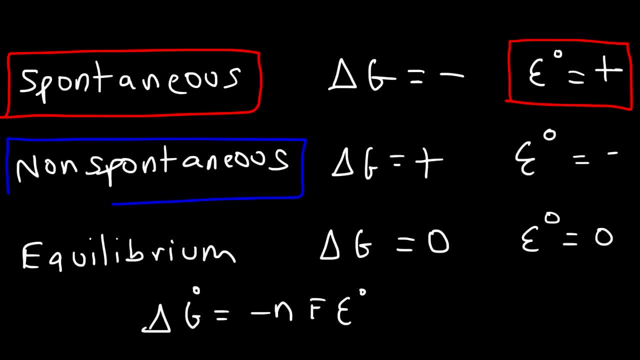 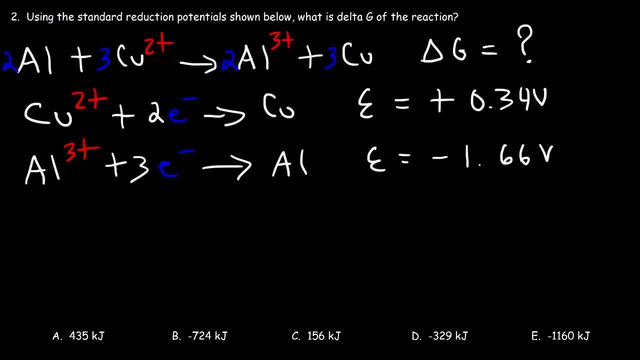 And for a non-spontaneous process in the forward direction, the cell potential is negative. So those are some things that you want to keep in mind. Number two: Using the standard reduction potentials shown below, what is delta G of the reaction? 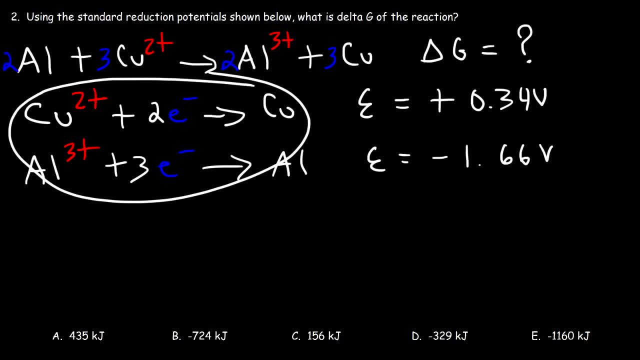 So somehow we need to combine these equations such that it adds up to this one, And we need to get the cell potential for the overall balance reaction and then, once we have it, we can calculate delta G. So notice that aluminum is on the left side. 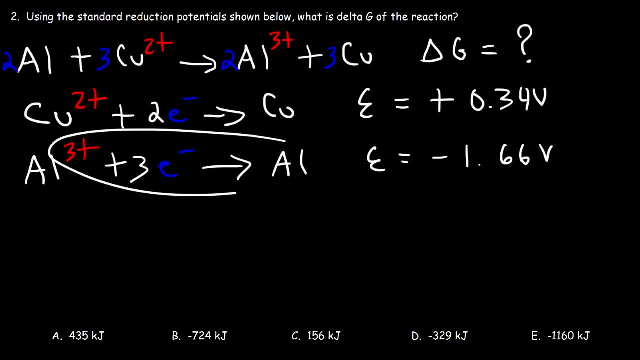 Copper is on the right. So that indicates that we need to reverse this reaction, And for this one, copper is on the appropriate side. Now we need the number of electrons to be the same, So two times three is six. We need to multiply this reaction by two. 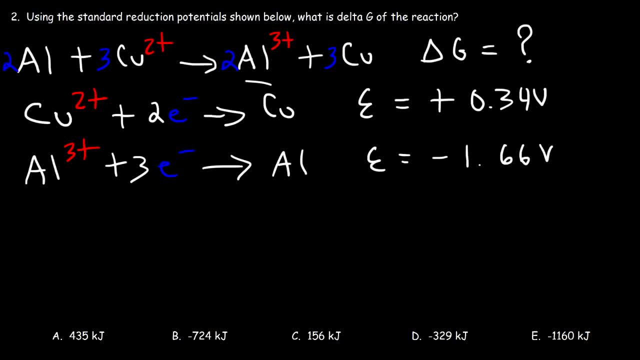 and that will give us two aluminum. And this one by three to get six electrons, which will give us three copper atoms. So let's reverse this reaction and multiply it by two. So it's going to be two A, two B and two C. 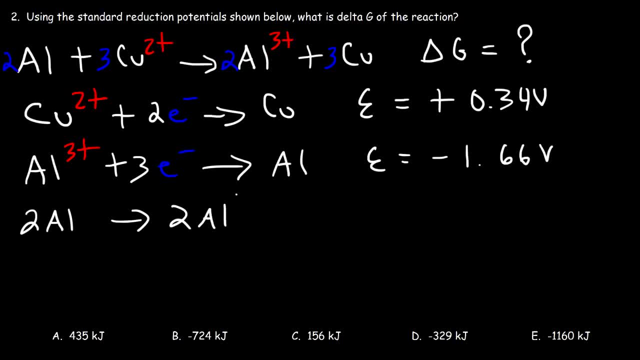 And that turns into two Al three plus with six electrons. Now, if you reverse the reaction, the cell potential will change from negative to positive. If you multiply it by two, it has no effect on the cell potential. Now, this one, we're not going to reverse it. 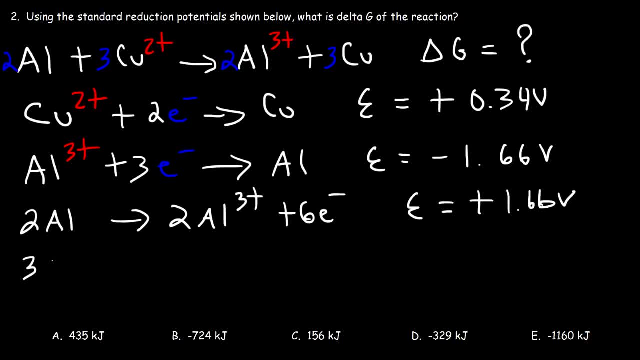 but we're going to multiply it by three, So we're going to have six electrons And the cell potential will not change. It's going to be positive 0.34 volts. So now let's add up these two reactions. Notice that the electrons will cancel. 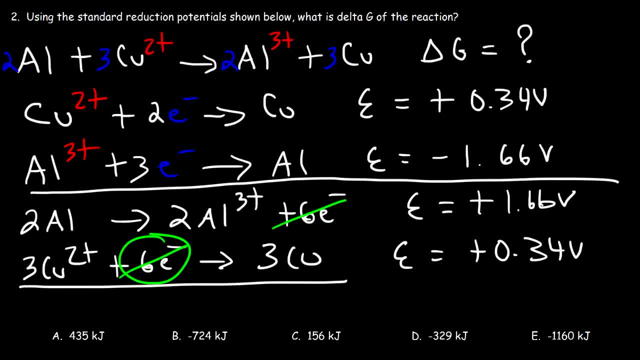 We have six on the left and six on the right. If you subtract both sides by six, they both disappear, And so this will give us the net reaction which is what we have here. So now we can get the overall cell potential for the entire reaction by adding these two values. 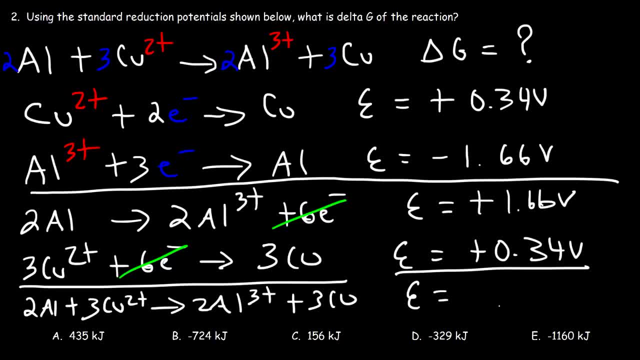 1.66 plus 0.34 is two volts, And we can see that N is equal to six. So now we can see that N is equal to six And we can see that N is equal to six, And we can see that N is equal to six. 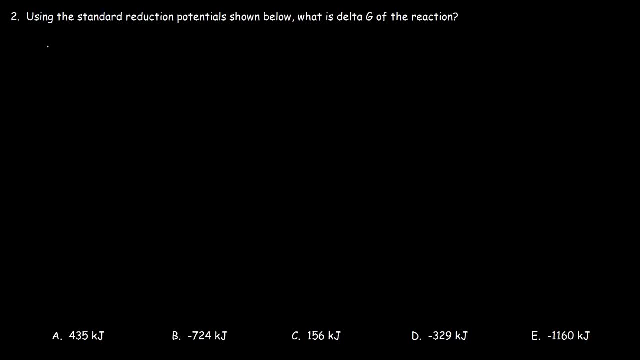 So now we can calculate delta G. So the cell potential for the overall reaction is two volts. N is six And we know that delta G is equal to negative N times, Faraday's constant times, the cell potential. So we have six moles of electrons. 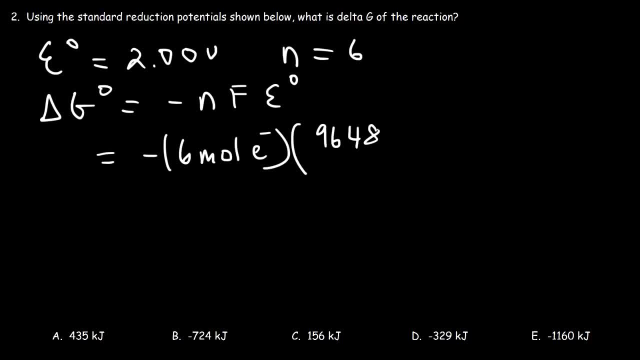 And Faraday's constant 96,485 coulombs per mole of electrons, And the cell potential is two volts or two joules per coulomb, And so this will give us delta G in joules, And so delta G is going to be negative. 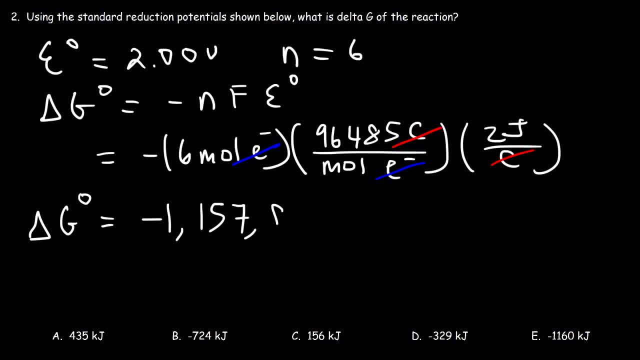 1,157,820 joules. Now let's convert that to kilojoules by dividing it by two, So you're going to get 11.55 by 5,000.. And so this is going to be negative 1157 .82 kilojoules. 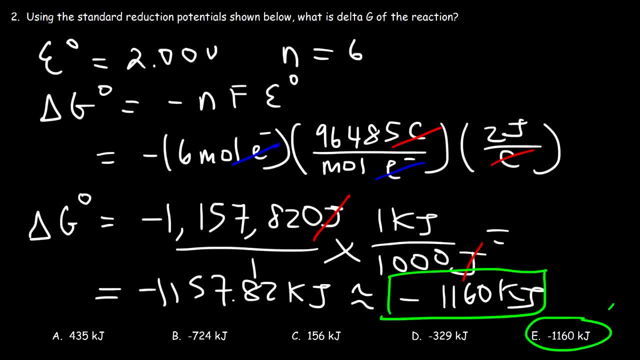 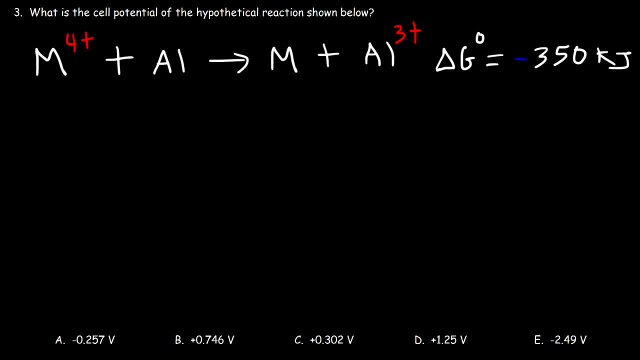 So we can round it and say it's about negative 1160 kilojoules And so that's the answer. This corresponds. what is the cell potential of the hypothetical reaction shown below? now, if you want to try it, go ahead. pause the video now, the first thing we need to do. 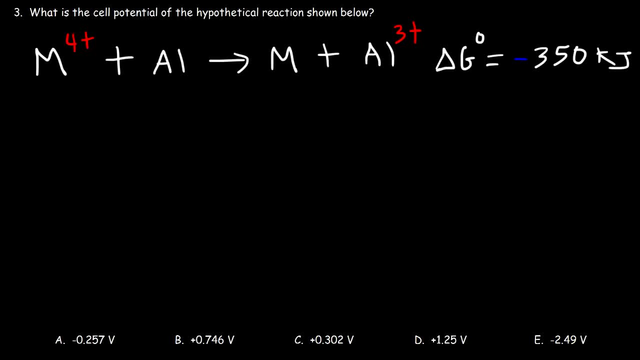 is we need to calculate n. we already have Delta G, and so once we can find the value of n, then we can calculate the cell potential easily. so let's focus on the first half reaction, where m4 plus turns into M, and so to balance it, we 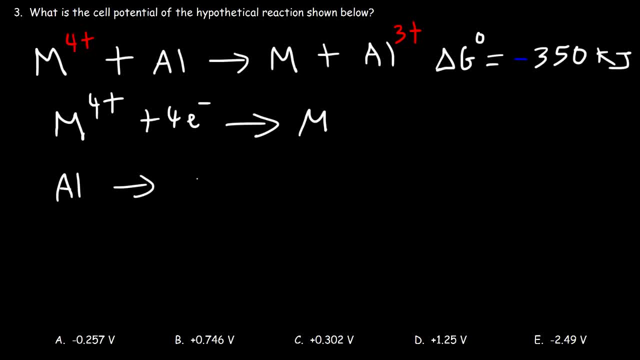 need four electrons. now for the second half reaction, we need three electrons, and to make the number of electrons equal 4 times 3 is 12. we need to multiply this by 3 and this by 4, and so in both cases we're going to get 12. 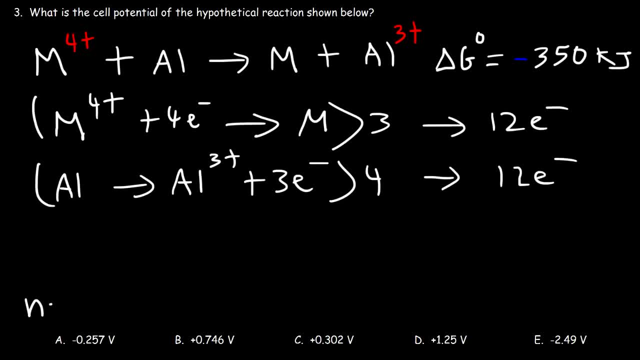 electrons. so clearly we could see that n is equal to 12 for this example. so now that we have the value of n, we can calculate the cell potential. now, before we use the equation, we need to convert this to joules. so we have 350 kilojoules and we have to multiply it by a thousand joules per. 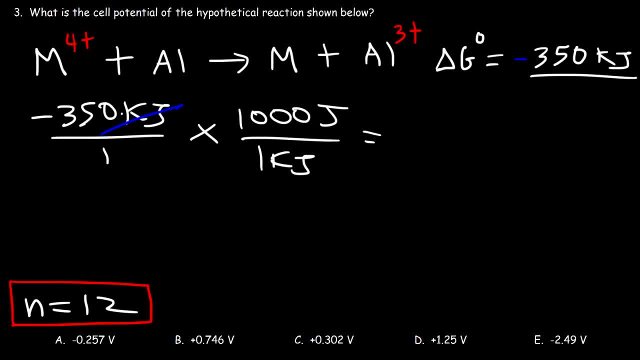 kilojoule to convert it. so this is the same as negative 350 thousand joules. now we can use this equation. so Delta G is negative 350 thousand joules and we know it's 12. Faraday's constant is ninety six thousand four hundred. 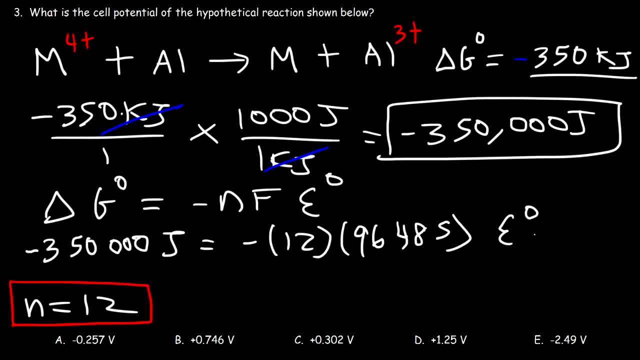 eighty-five, and let's solve for the cell potential. so all we need to do is divide both sides by negative 12 and ninety six thousand four hundred eighty five, type in negative 350,000 and divide that by negative 12 and then take that result, which is 29 thousand. 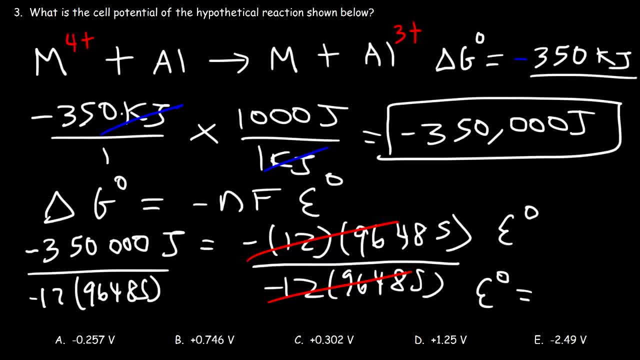 one hundred sixty-six point seven. divide that by ninety six thousand four eighty five, so you should get positive three zero to volts and that's the answer. so that's how you can calculate the cell potential. if you're given lance AC, you need to calculate the number of moles of electrons and the balance of Undσι accumulate. but this is an even calculation. so what we do, when we take the information out of the answer and the number of profit coming when you change into g, are more or less for profit as an cancellation of p and in fact isn't considered positive. positive, yes, I'm defeat if you use the equation across both the numbers degli increasing. 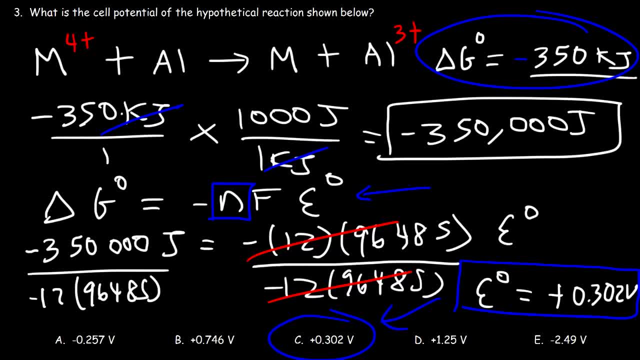 rando dos is that 7 x plus x the seen. if a number of electrons more or less than 20 in each other, then doesn't give down 12. if you use same price way and multiply that, I'm doing ok and a balanced chemical reaction, and then you could use this formula. So that's it for this video. Thanks again for watching.